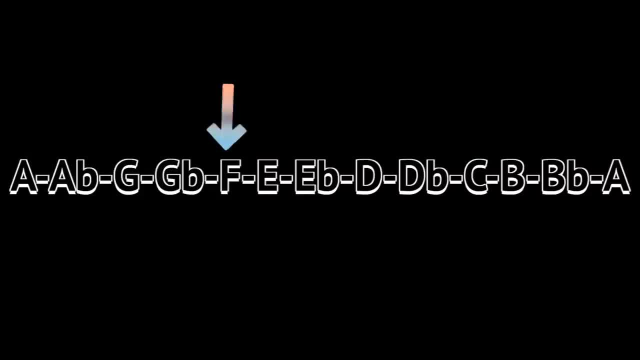 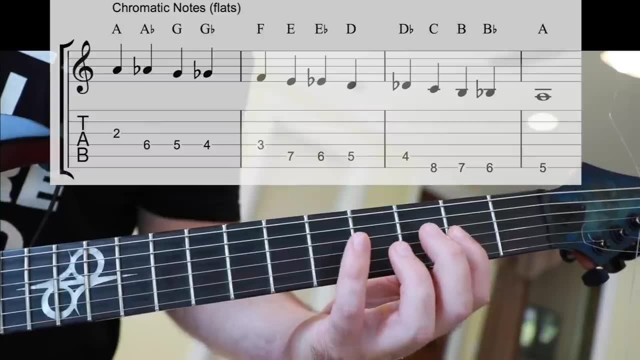 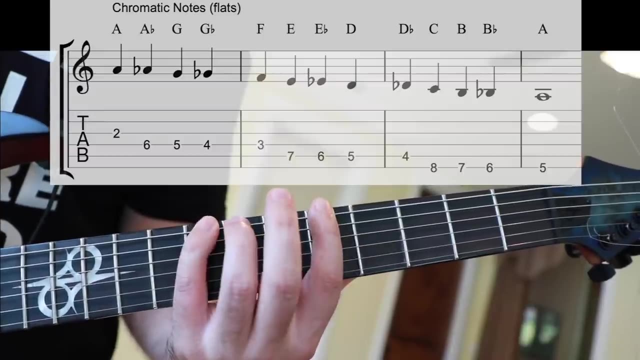 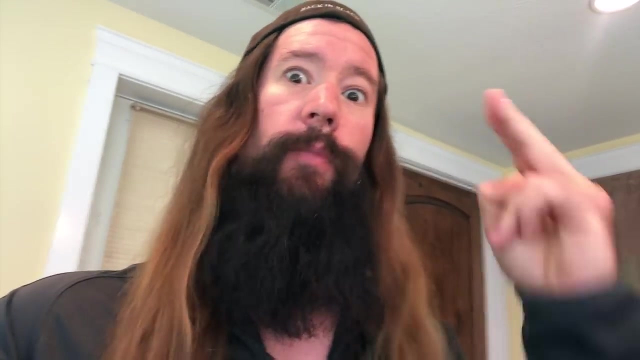 A, A flat, G, G flat, B flat, F, E, E flat, D, D, flat, C, B, B flat and A. Now I've been hitting you guys with a lot of information. One thing I find that helps increase brain power is to get a pump. 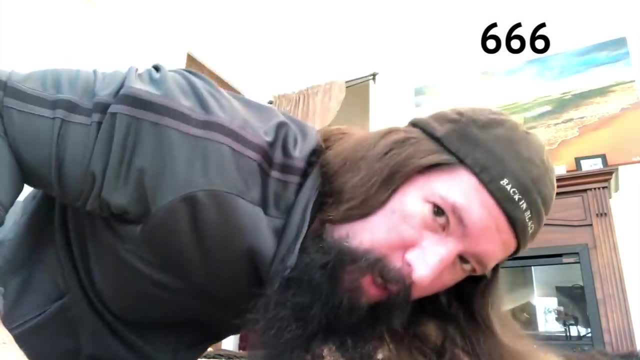 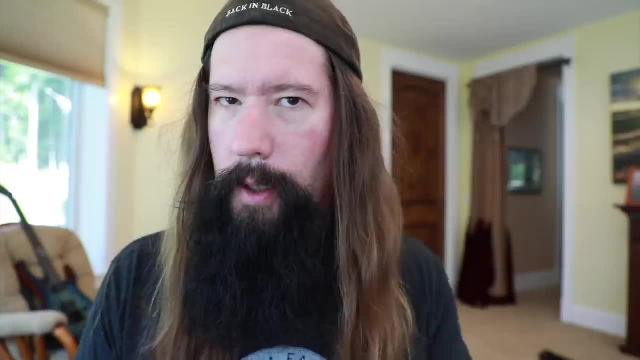 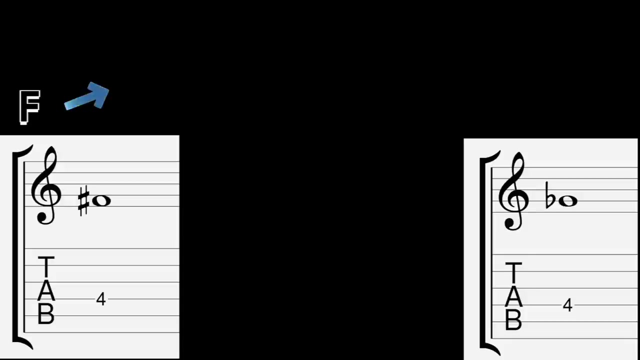 665, 666, 667.. 668, 669.. Now here's the trick. This F sharp note is the same as G flat. By raising an F, we get F sharp. By lowering a G, we get G flat. 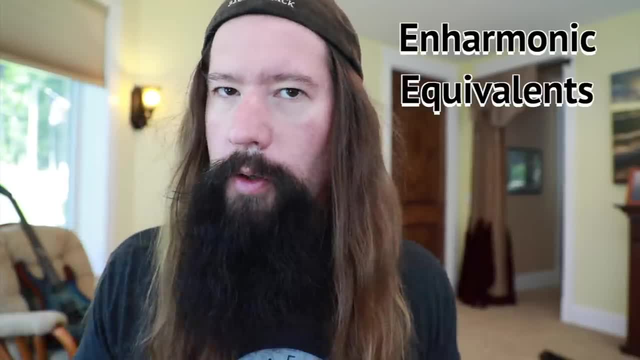 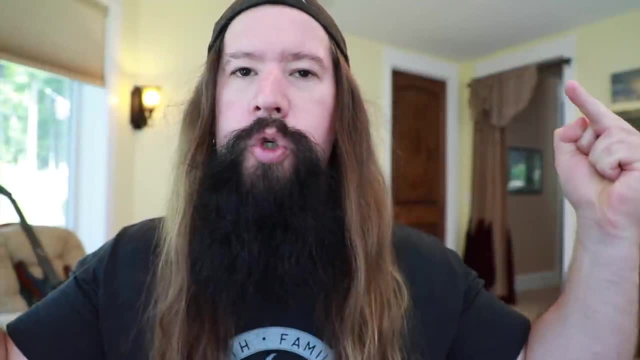 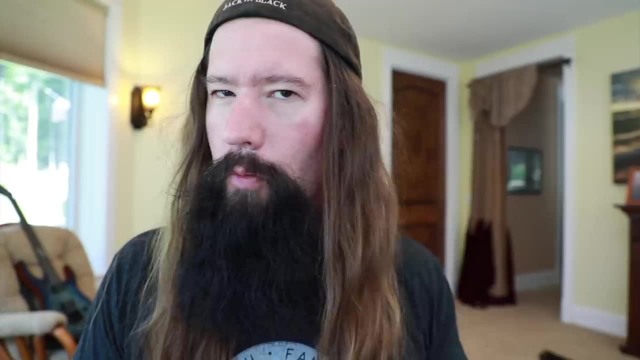 Same note, two different ways to label it. Now, you can do this with any sharp or flat, And the concept is called enharmonic equivalent Pfff. What is a scale? Now, I'm not checking to see how fat you are. 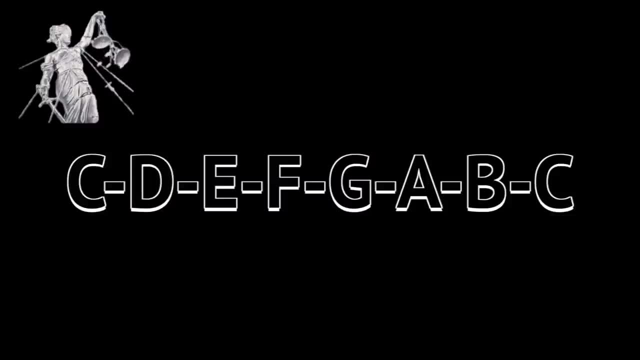 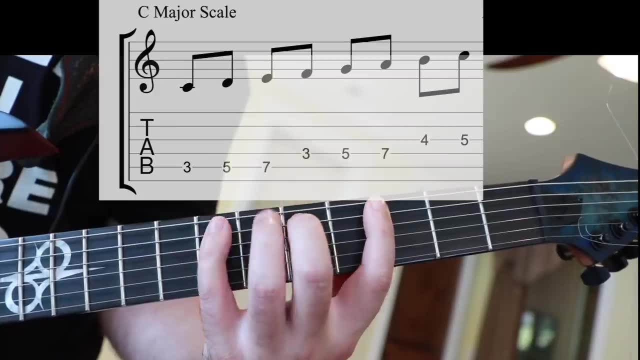 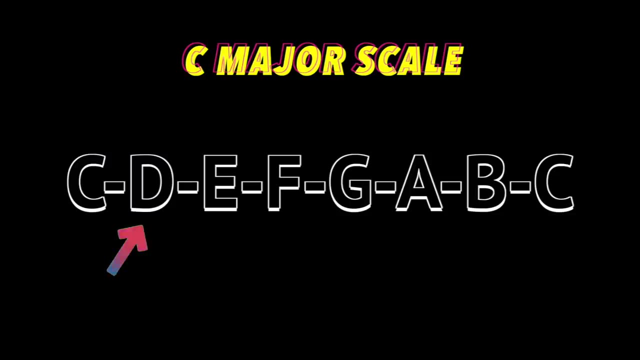 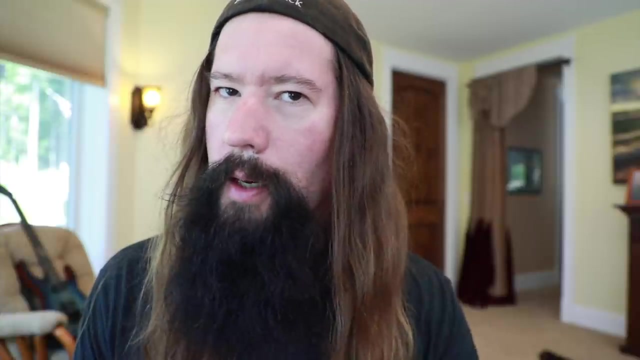 I've become quite large. A musical scale is just a series of notes connecting an octave. Here's the C major scale. The C major scale contains the notes C, D, E, F, G, A and B. There's a formula you can use to generate any major scale. 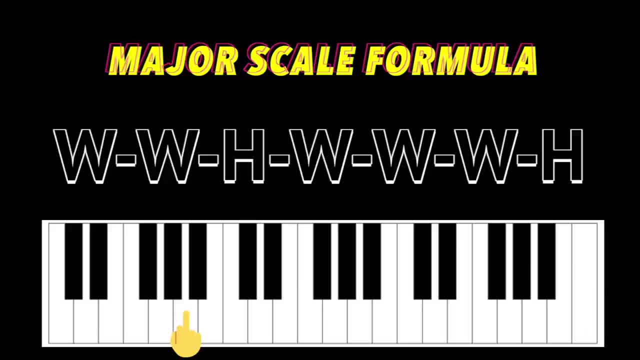 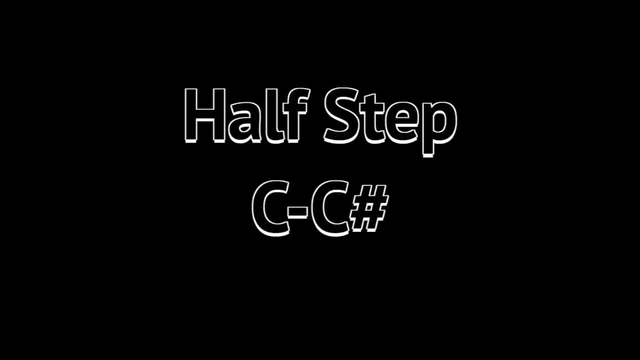 Whole step, whole step, half step, whole step, whole step, whole step, half step. Here's how it works. A half step is from C to C sharp, or one fret on the guitar. A whole step is from C to D, or two frets on the guitar. 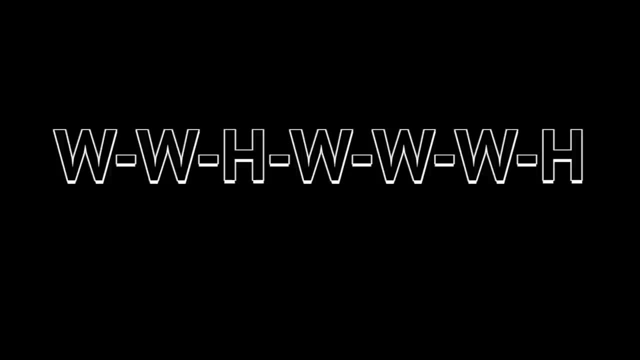 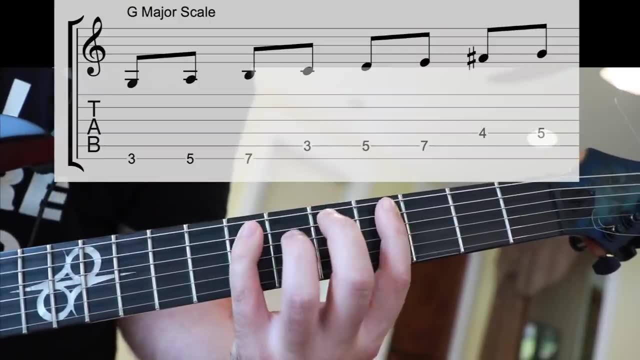 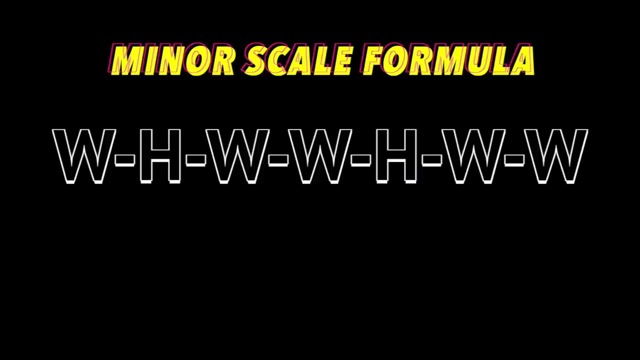 Use this formula: starting on any note to make a major scale. Start on the note G to make a G major scale. To make a minor scale, use the formula: whole step, half step, whole step, whole step, half step, whole step, whole step. 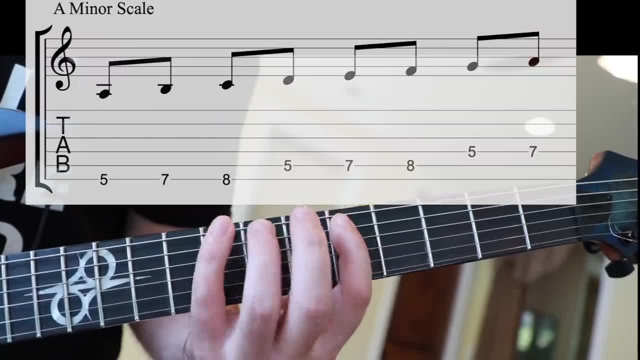 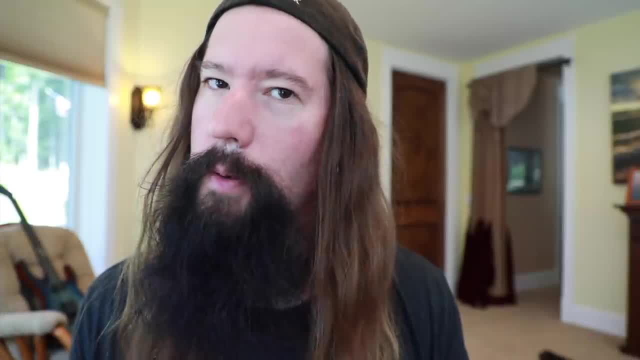 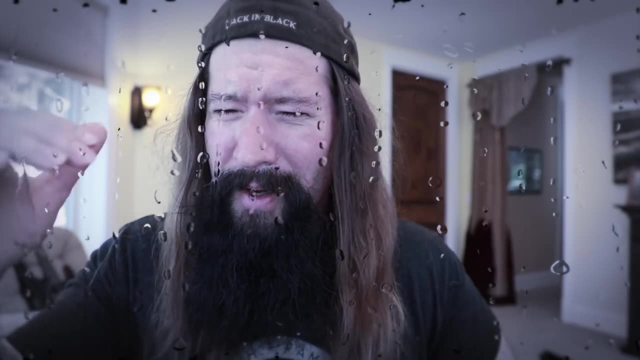 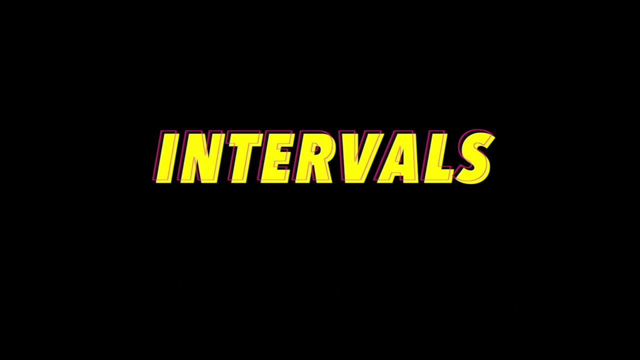 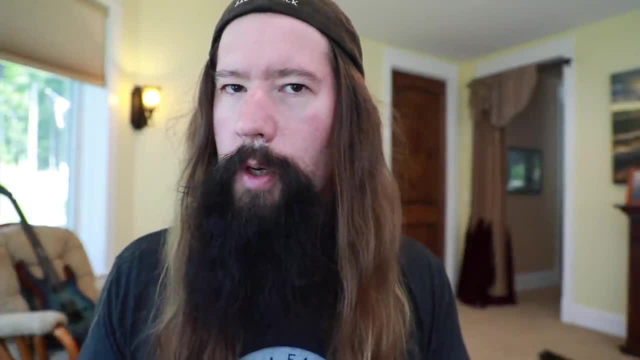 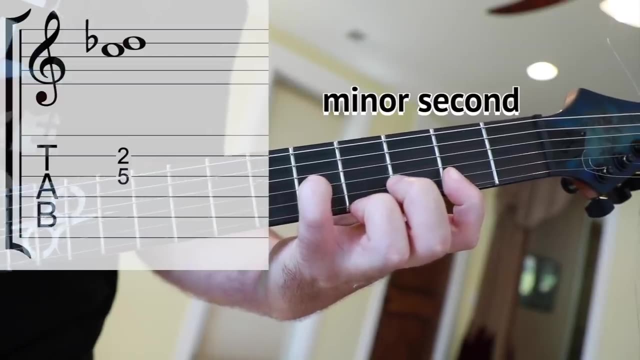 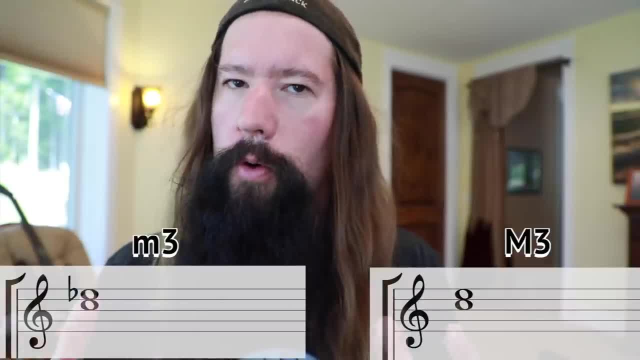 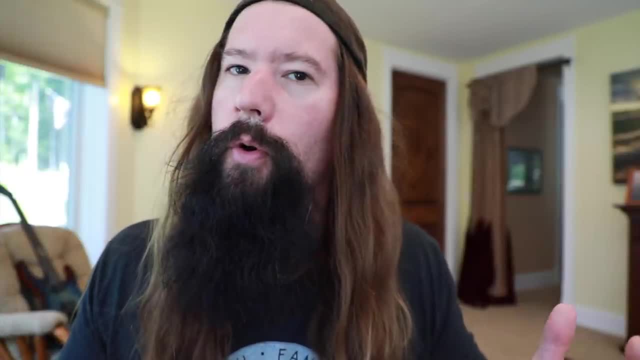 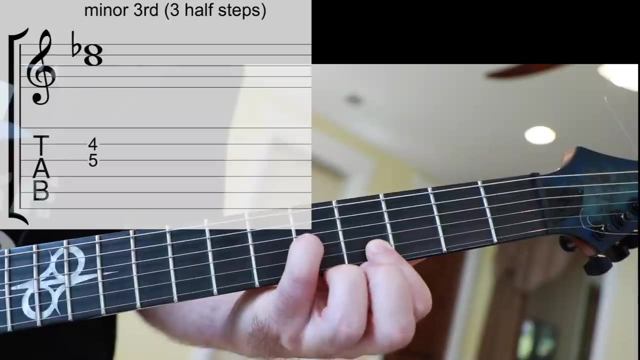 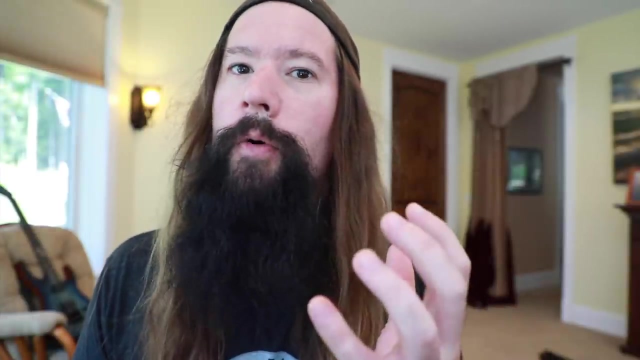 The most important intervals to know are the thirds, because those dictate the tonality of chords. If you're in a happy mood, try a major third. Let's dash those dreams with a minor third. That's better. By the way, you can now get my evil laugh as a ringtone. 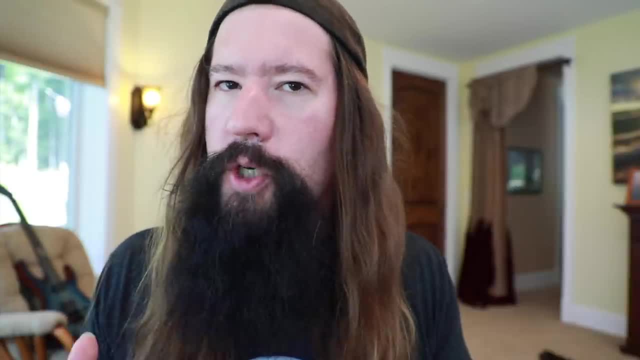 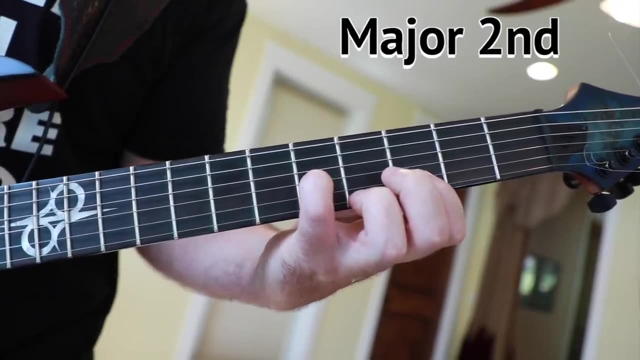 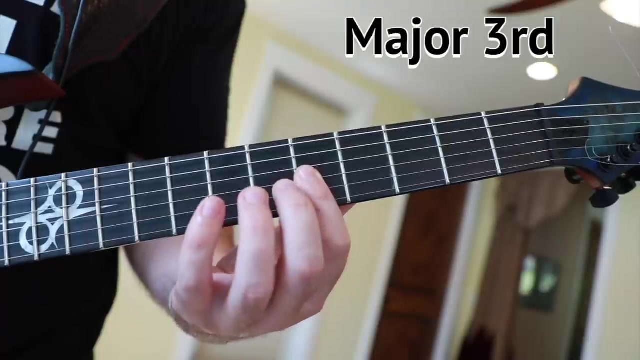 I'll leave a link in the description below For the overachievers. here's all of the intervals within the octave. So you just gotta put your fingers up and open your fingers up and you're all set, And I'll leave that up to you. 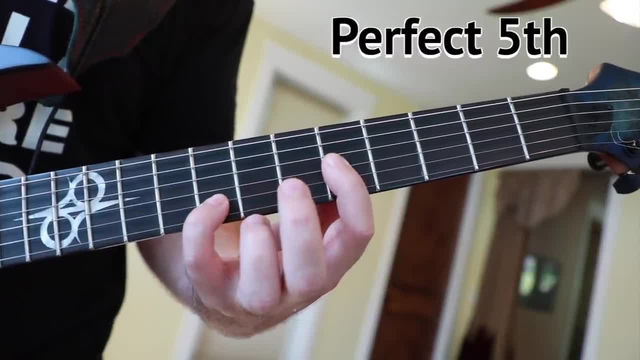 I'll let you know all the intervals and I'll let you know the rest later. I think there's just one more thing I'd like to say. I know I was a little too hard on you. I know I was too harsh. 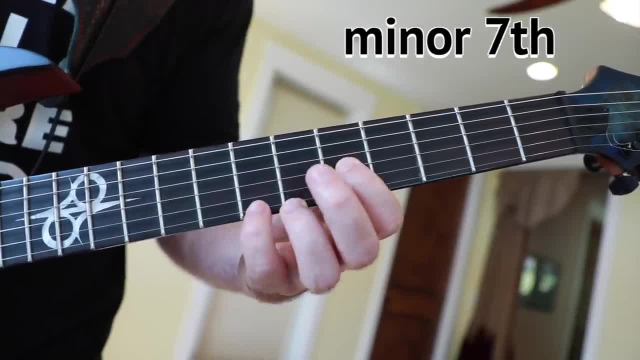 I know I've been overreacting, but I'm out of control. I'm gonna have to say something. I'm not thinking we're in the same boat. I'm getting used to it. I don't think I've ever been the same in any of the classes these days. 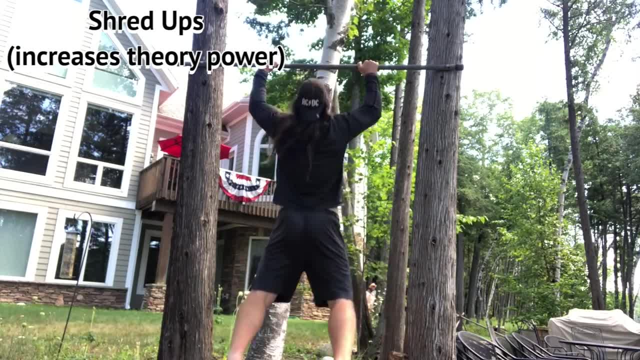 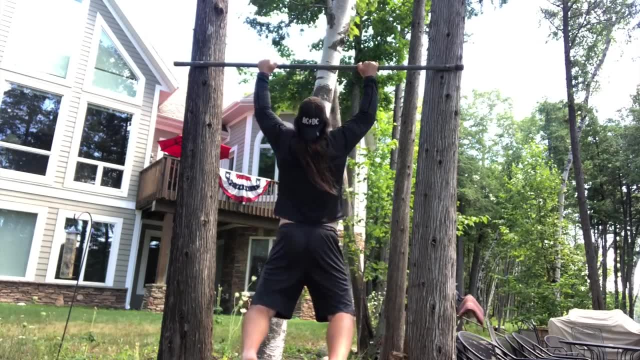 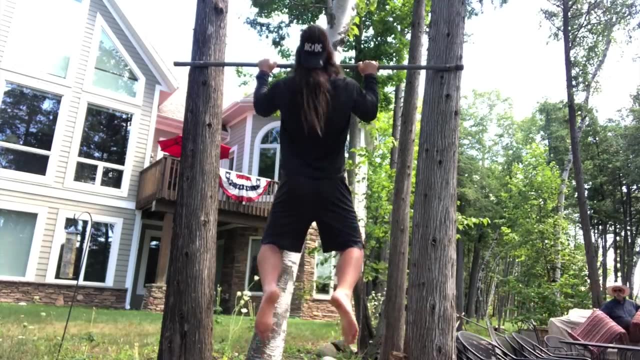 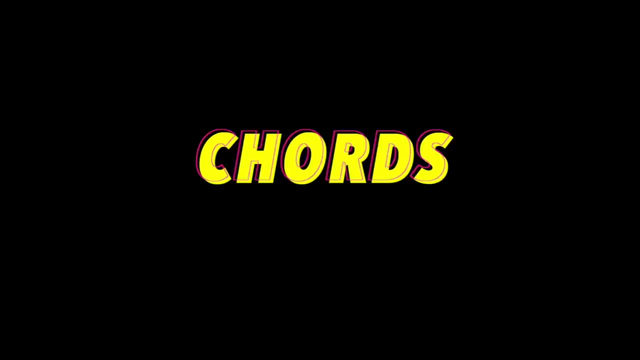 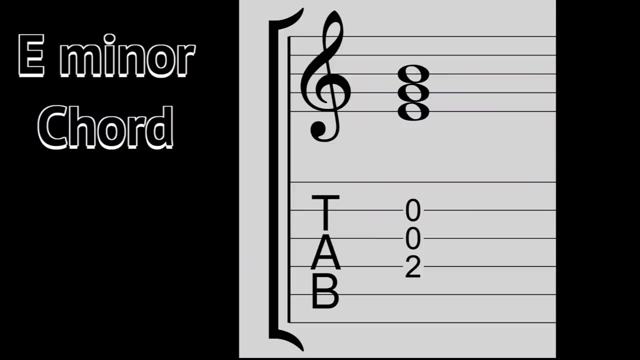 I'm just gonna go back and have a little rest, So if you need help, please let me know. See you next time. Chords are three or more notes played together. I'm a huge fan of chords because they communicate such a powerful range of emotions. 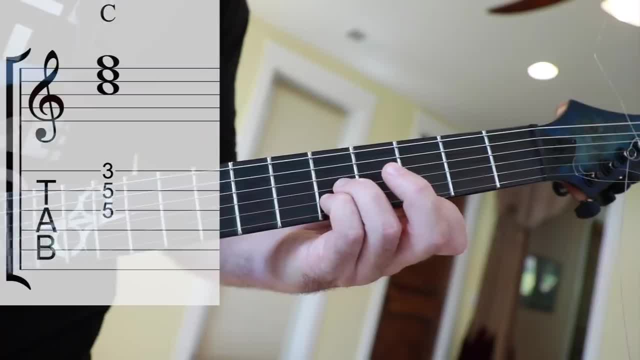 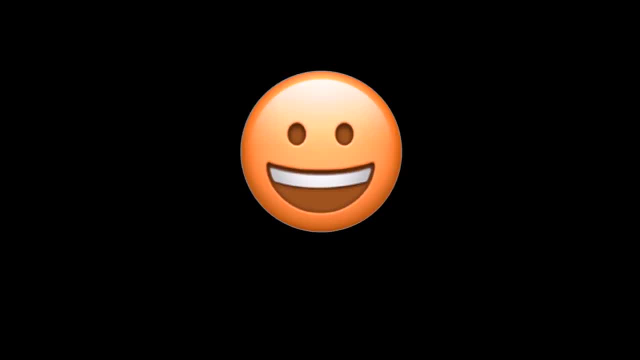 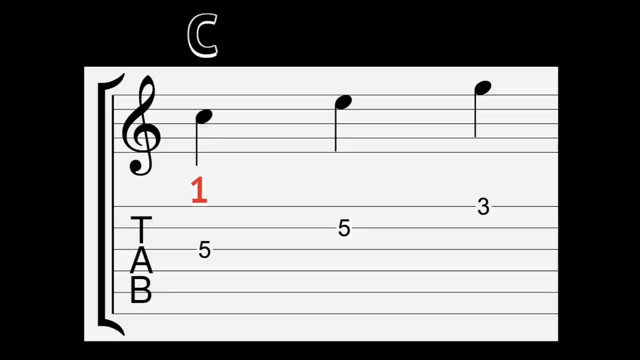 Major chords produce an uplifting quality To make a major chord play the 1,, 3, and 5.. In other words, C is the 1,, the 3 is the major 3rd E and the 3 is the major 3rd B. 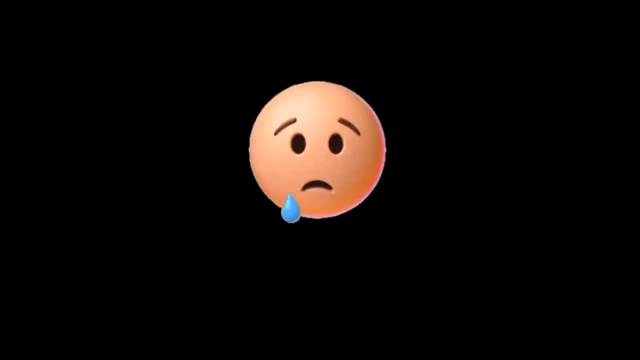 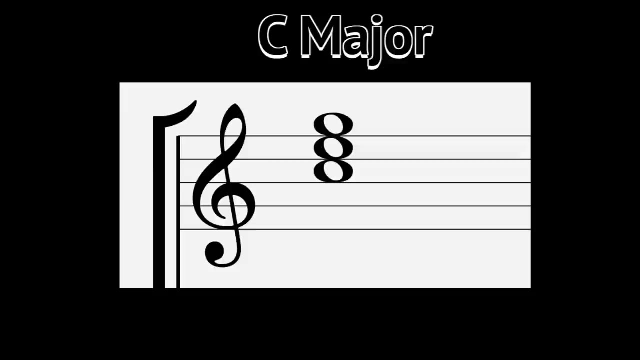 And the 3 is the major 3rd. E And the 5 is a perfect 5th. G. Spoil the party with some doom and gloom by playing a minor chord. All you have to do to a major chord to make it minor is flat. the 3rd. 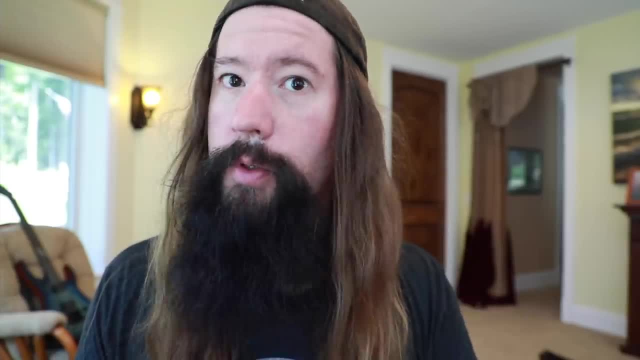 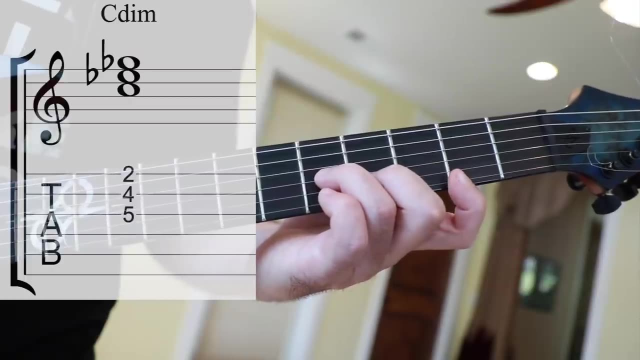 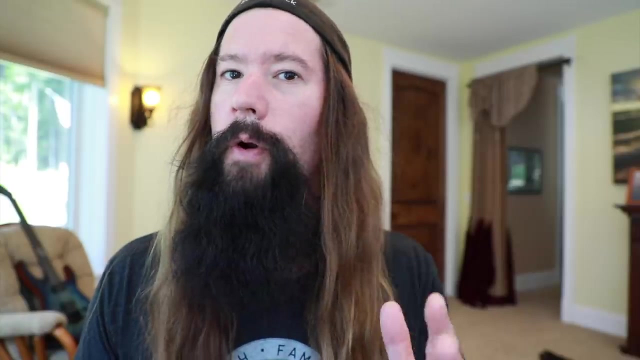 Now there's just two more basic shapes to know about when it comes to chords: The diminished chord. Ooh, very scary Flat. the 5th of a minor chord. A minor chord to make it diminished. This is a very important chord for metal and classical music. 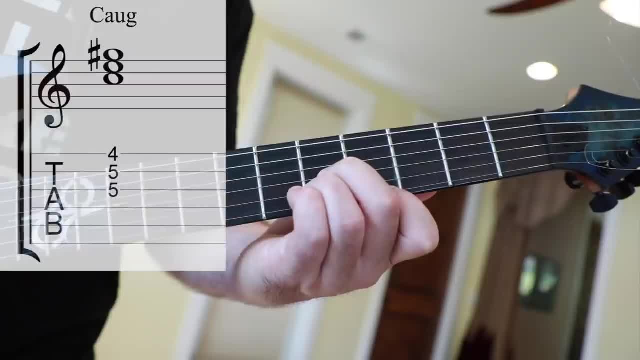 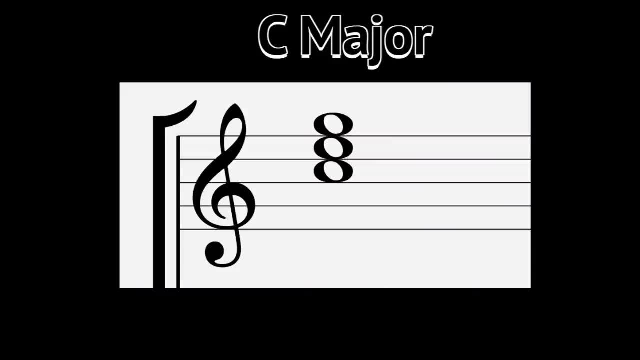 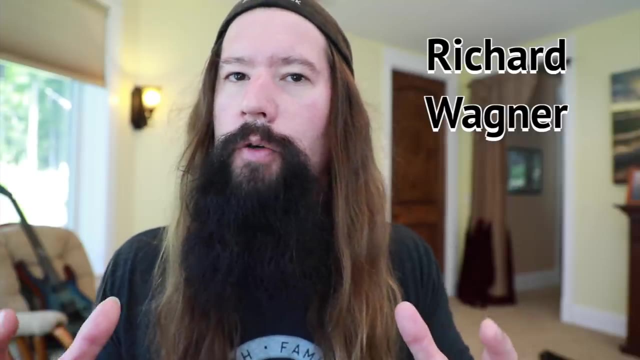 And finally we have the augmented chord, A very creepy sound used in horror movies. Just raise the 5th of a major chord to score an augmented triad. You can hear this chord in Richard Wagner's Ride of the Valkyries. 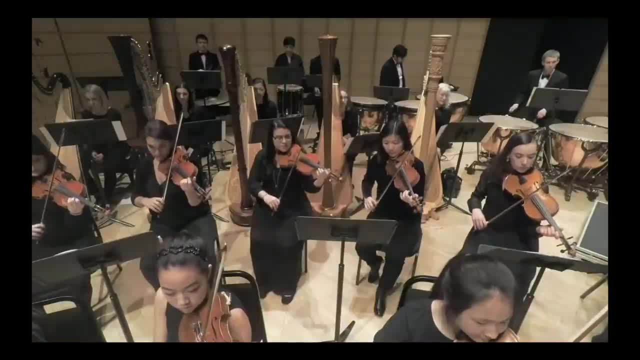 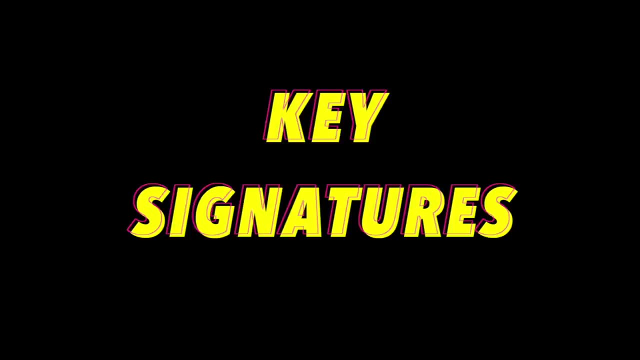 A very creepy sound used in horror movies. A very creepy sound used in horror movies. A very creepy sound used in horror movies. Just raise the 5th of a major chord to a minor chord. You can hear this chord in Richard Wagner's Ride of the Valkyries. 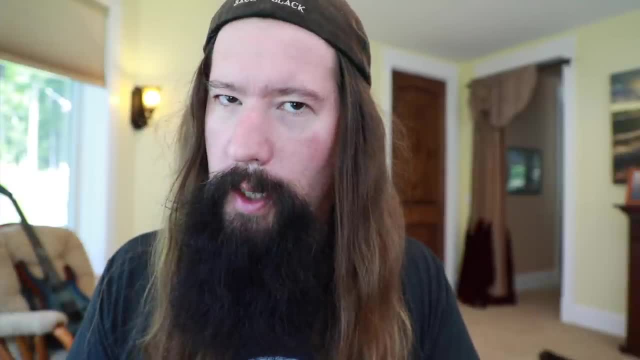 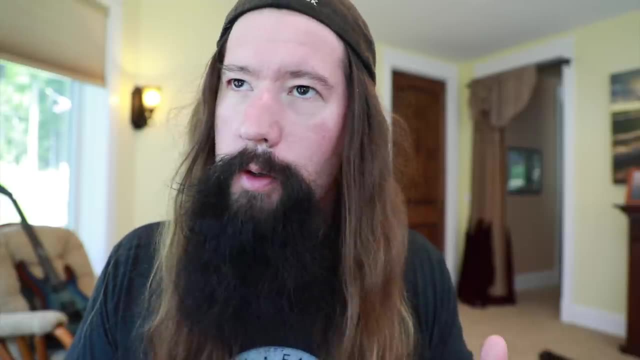 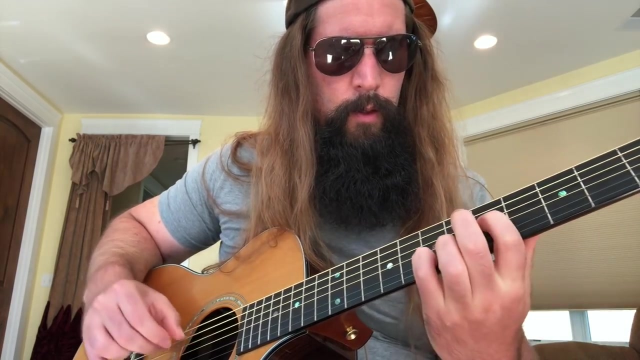 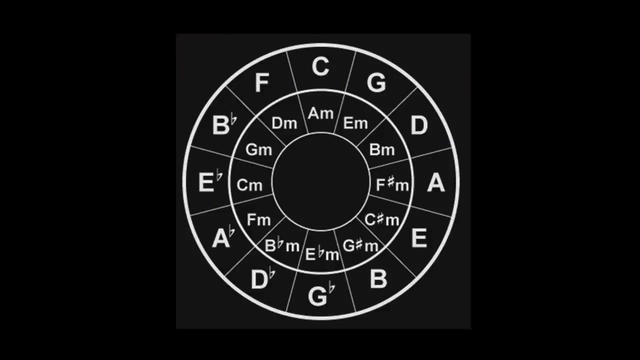 Key signatures tell you what notes are in each key. The circle of fifths is a diagram that illustrates each of the 12 musical keys. Before I understood keys, I used to sound like this: yes, here's how it works. at 12 o'clock you have the key of c, with no sharps or flats. each time you 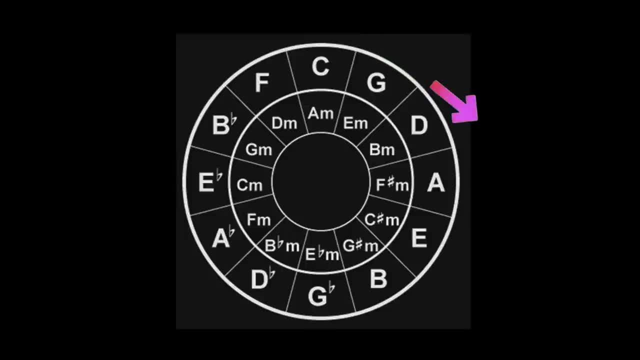 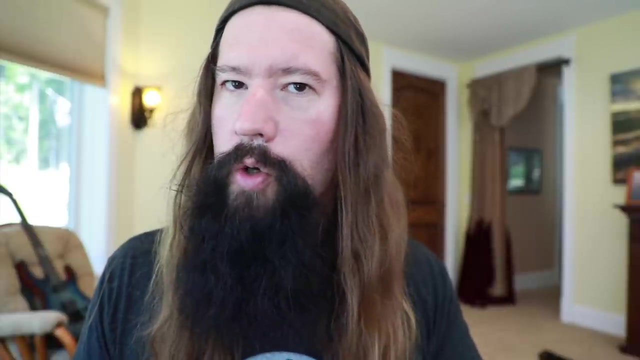 move clockwise. you go up a fifth in the musical alphabet: c, d, e, f and g. so our next key after c is g, after g, find the next key by going up another fifth: g, a, b, c, d and thus d is the next key. d stands for damn. i love music theory and that's why it's called the circle of fifths, because each 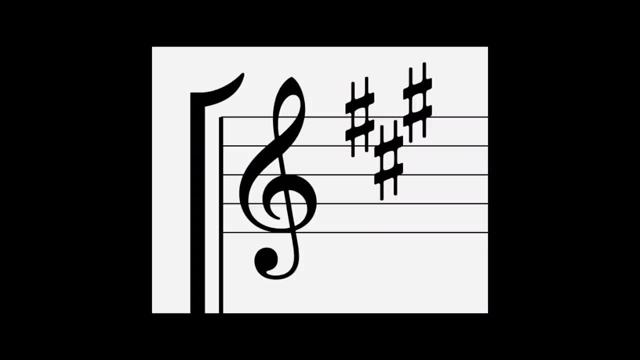 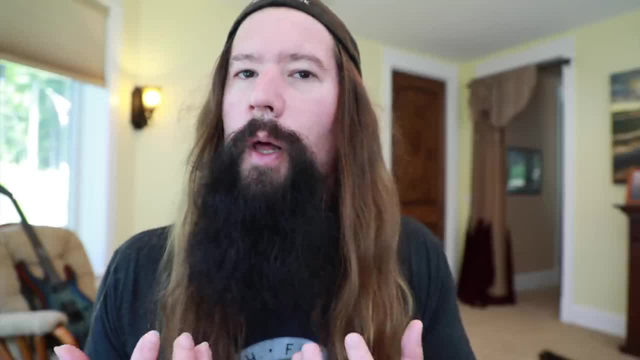 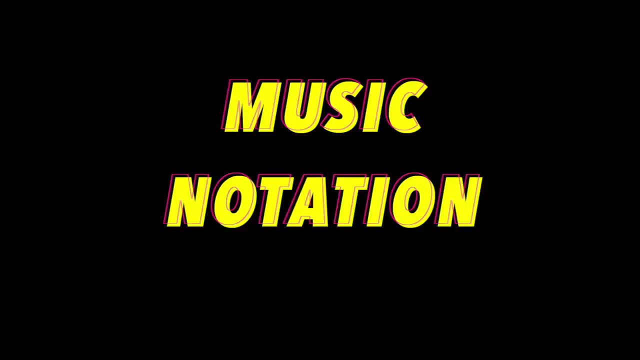 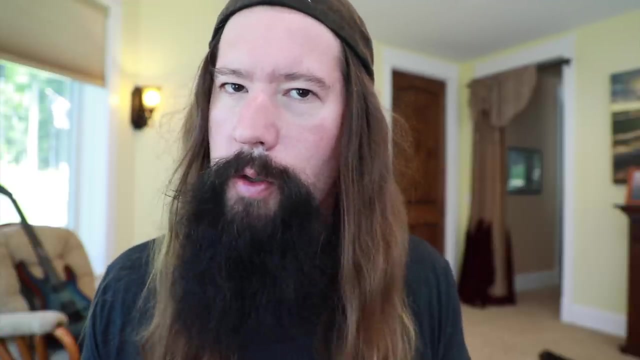 key is five notes apart. the sharps found in each key are also a fifth apart: f sharp, c sharp, g sharp, and so on. once you internalize this circle, making sense of the music you hear becomes a lot easier. now being able to read music doesn't make you a real musician or anything, but it does make it. 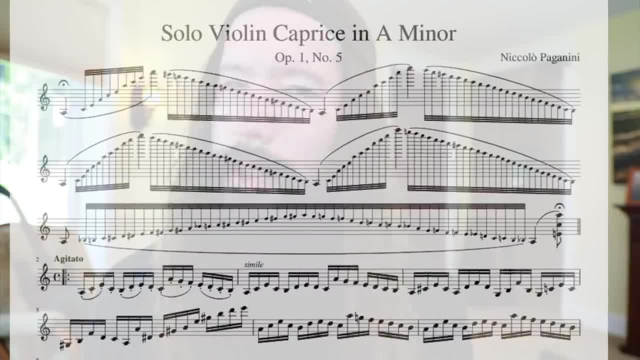 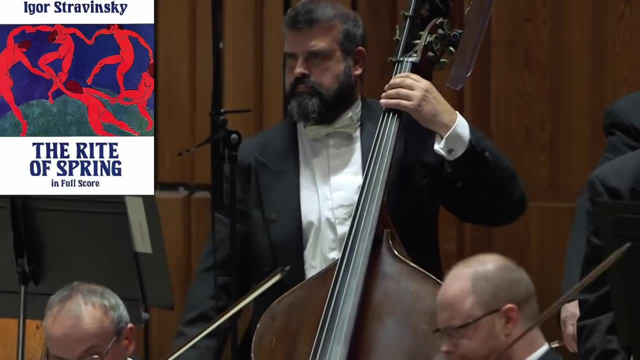 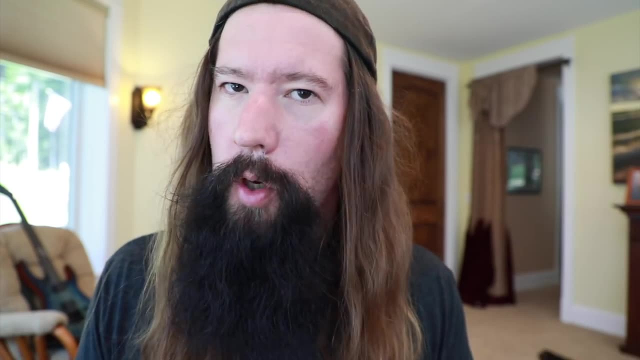 easier to absorb musical ideas, and that's why i'd recommend all musicians work on their reading jobs, myself included. if you ever want to learn how someone like igor stravinsky or john williams orchestrates their music, reading is a must. now here's the notes on the staff: e, g, b, d and f are the notes on the lines try using. 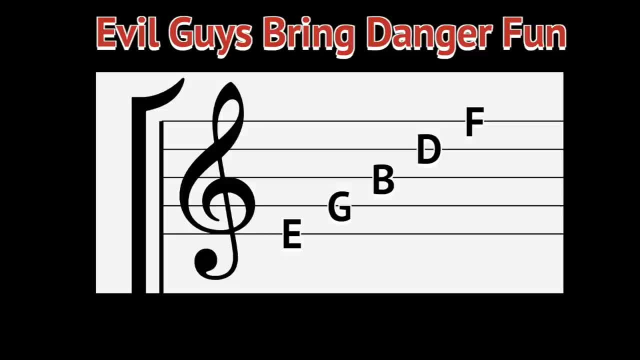 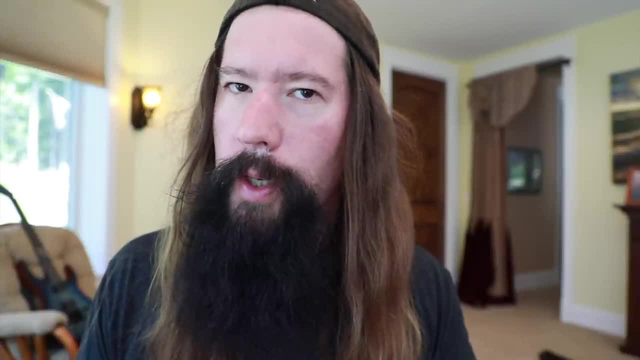 the acronym evil guys bring danger. fun to remember them. the notes on the spaces are f, a, c and e, spelling the word face as in: i want music theory all up in my face, bro. now let's practice reading an evil version of twinkle, twinkle little star. 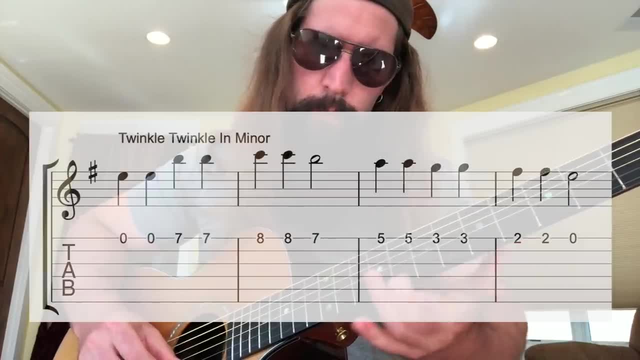 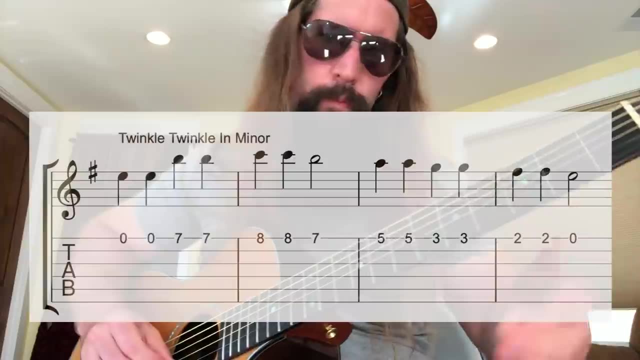 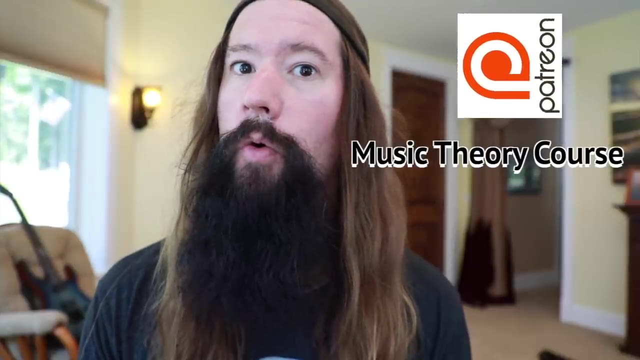 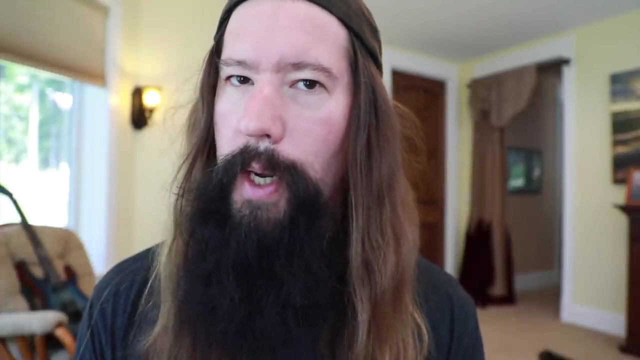 you can get more exercises for reading in my music theory course below. it only costs six hundred and sixty six dollars and that pretty much covers the basics of music theory. it's definitely not rocket science, but it does take some time to learn how to read music theory. so i'm going to show you. 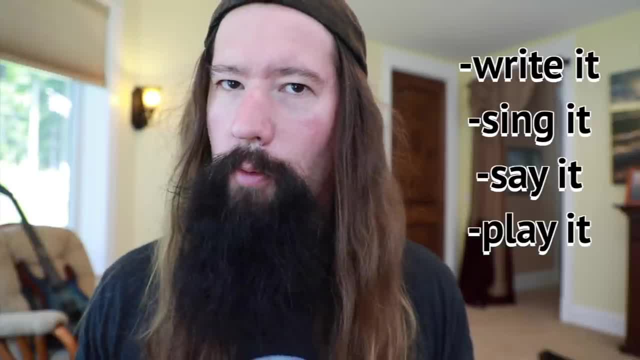 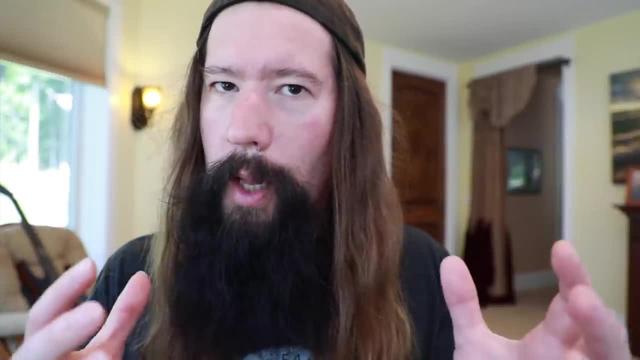 how to learn how to read music theory. and i'm going to show you how to read music theory and i'm going to wrap your head around. my music theory teacher used to say: write it, sing it, say it, play it, shout out to phil shackleton, and i really think that's true, confirming your knowledge from as many.